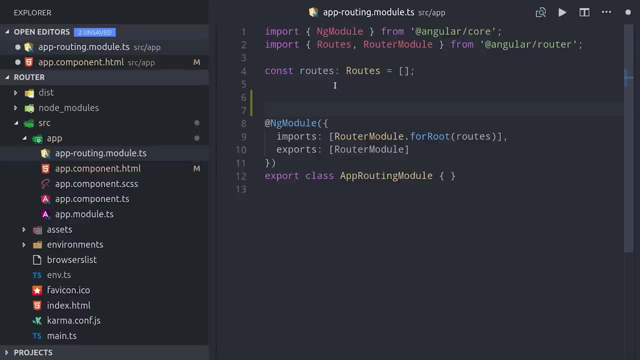 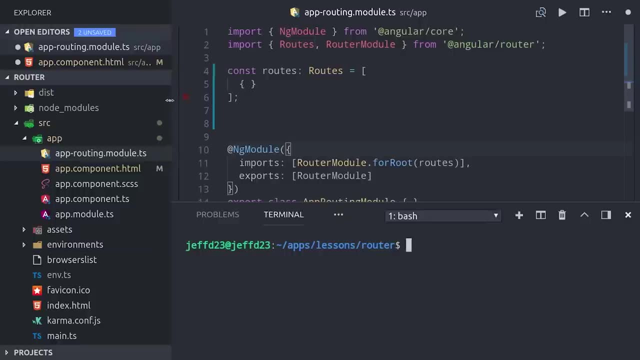 We can define each route in our application as an object, which will take a couple of configuration parameters. The most basic use case would be to give your route a path and then route it to a specific component that you've generated. Let's run ng: generate component. 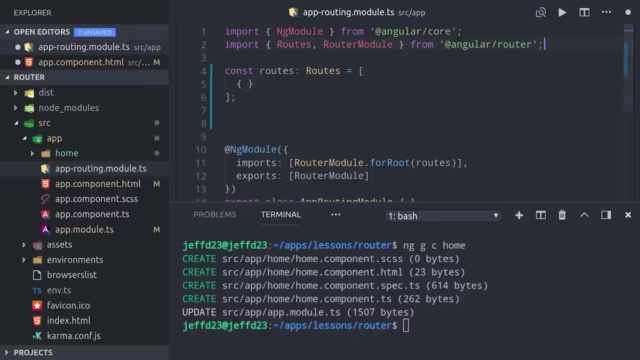 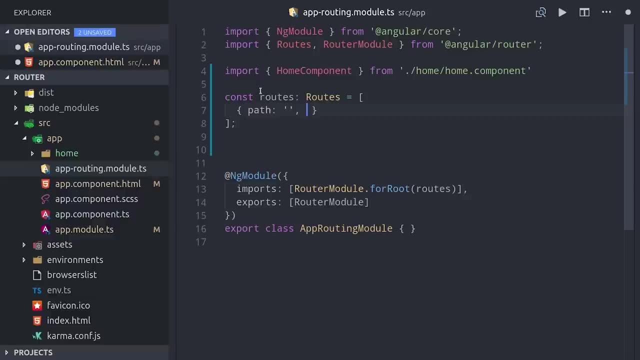 and we'll call this the home page. Now, the home page we could set up as the root path, so we'll give that a path. property of an empty string. then set the component option to the home component. If we serve the app, we should see the home component rendered. 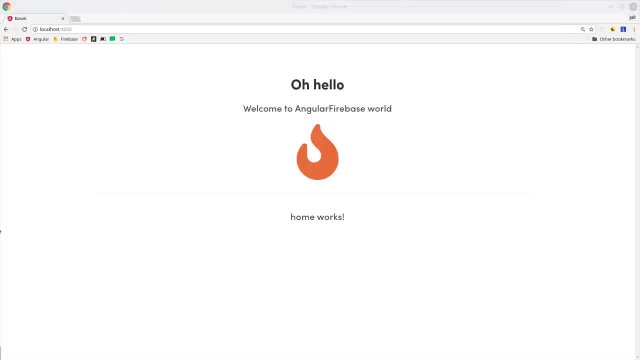 at the position of that router outlet. Then notice how other content in the home component is still there, such as the logo and the header. That'd be a good place to put a navbar and a footer and things that'll be present on every page. 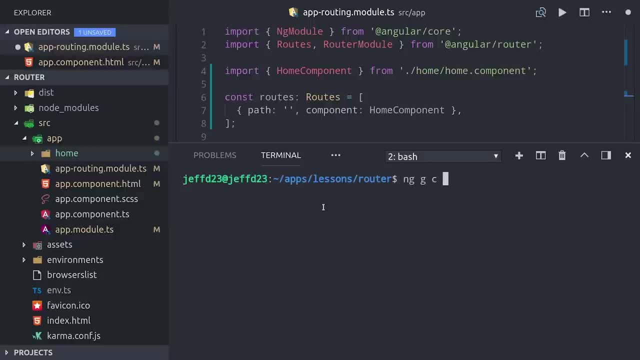 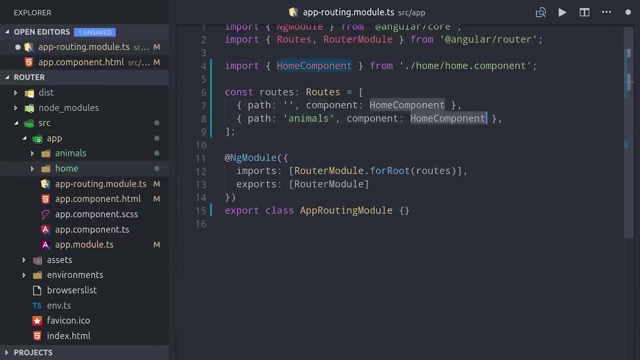 That's a good start, but let's look at how we can navigate between multiple components by generating another one called animals. Then we can import the component into our animal and set up another path and component property for this route. When setting up hyperlinks in Angular, you don't use a normal href attribute like you. 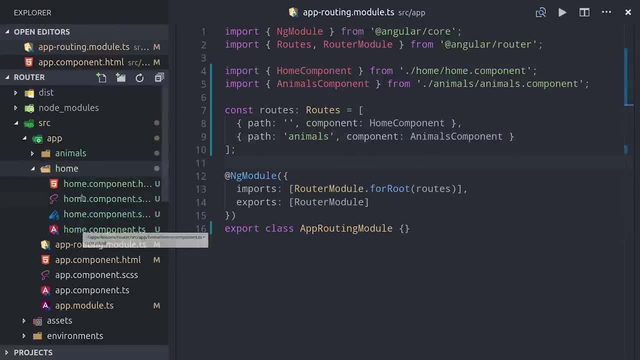 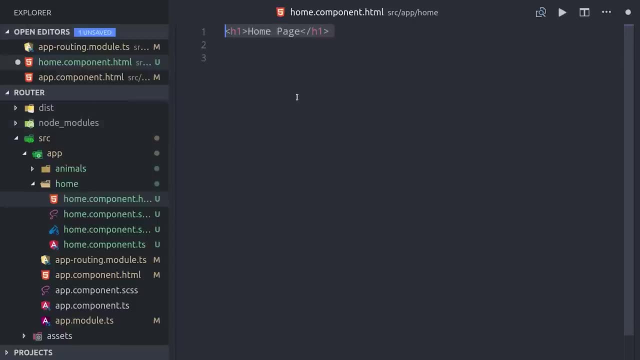 would in a plain HTML page. If you use a regular href, it'll cause your Angular app to completely reload whenever it's clicked. Instead we use the router link directive, which tells Angular to treat this as an internal route. Then we simply pass it the path that we would. 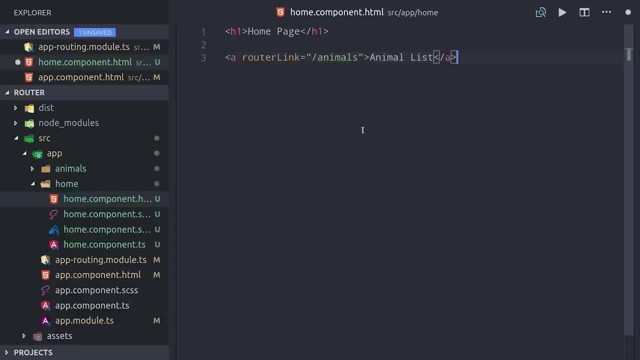 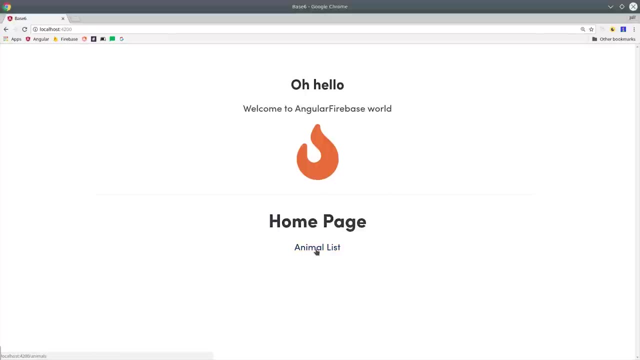 normally route to with a link. So now, if we open up the app in the browser, we can click on this animals link and it will route us to the corresponding component. So that takes care of your most basic use case. but what happens in the real world is: 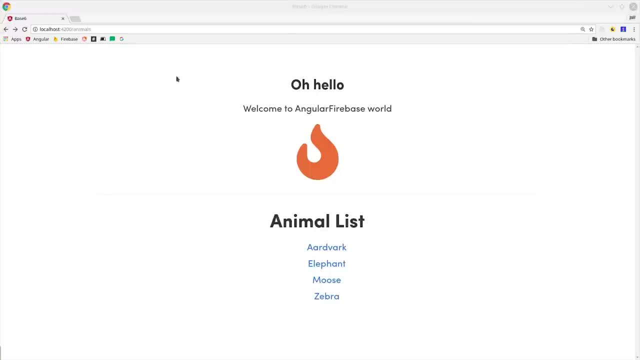 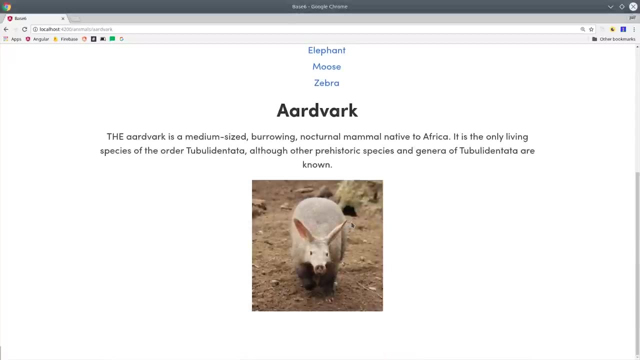 generally, you're pulling some information from a database, then route to a specific ID to show more information about that item, and you might have thousands or millions of items in your database, So you can't just hardcode all of those routes manually. In this next section we'll create a component called animal detail and we're going to make 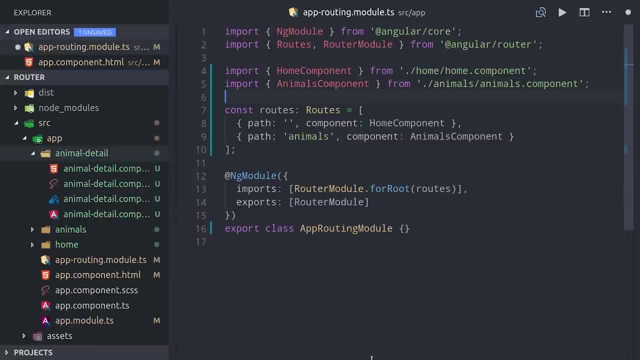 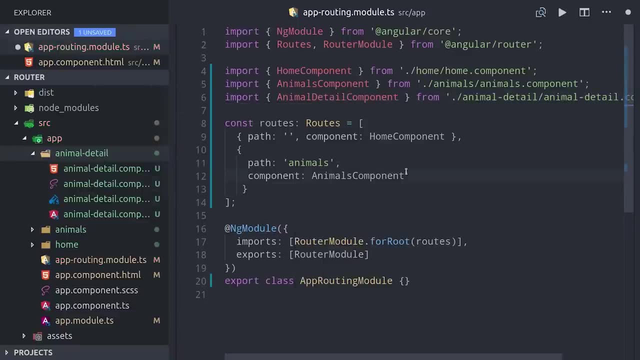 it a child route of animals. You can create child routes that will be rendered inside of their parent by adding the children property to the parent route, The children property itself will take an array of routes. so we just have a classic tree structure here. 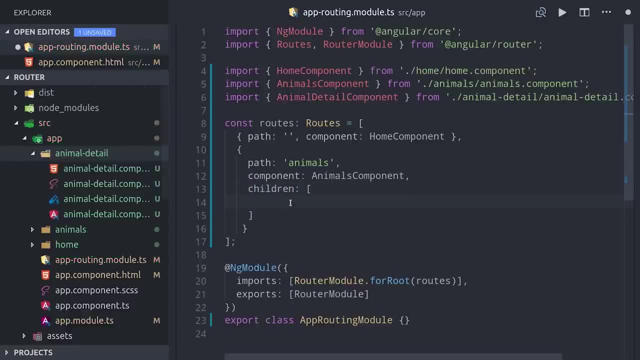 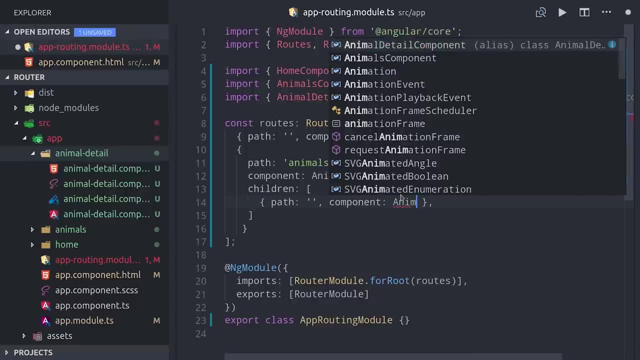 We can define a dynamic URL parameter by putting a colon in front of whatever that parameter is. In this case, we're going to be looking up animals by their name in our database, so we'll set up colon name as that URL parameter. Doing this means that we can navigate to routes that will look like animal slash elephant. 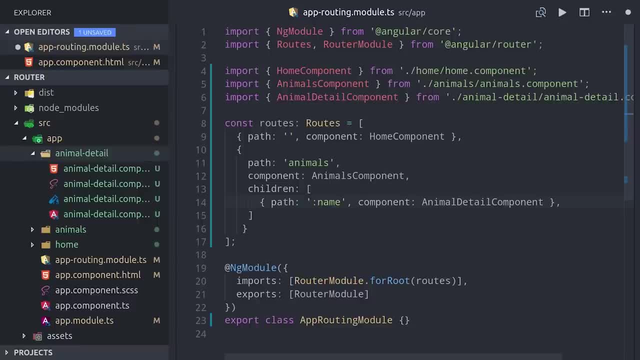 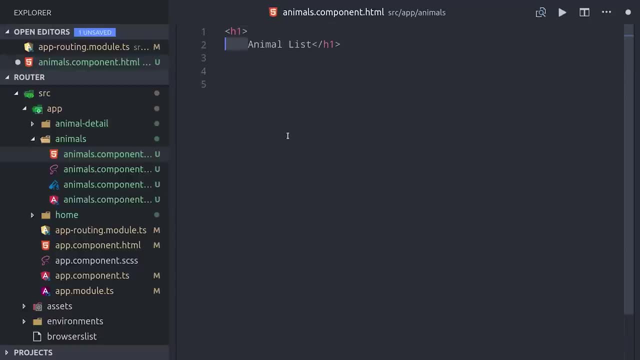 animal slash, aardvark or any other dynamic property that we pass to the second half of that URL segment. Notice that we're dynamically generating a list of links that we're pulling from Firebase, so let me show you how I do that. 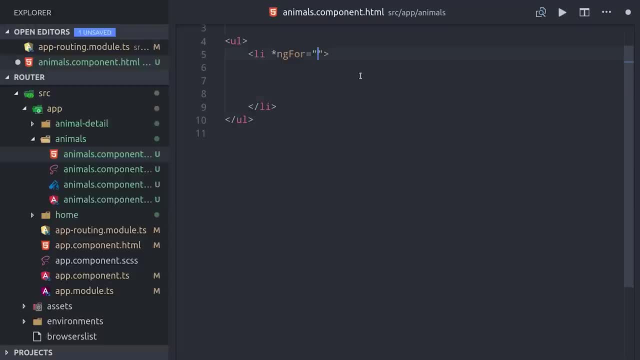 In the parent component I have an array of documents that I pulled from Firestore so I can loop over them asynchronously with ng4 and the async pipe. Then, to build the link, instead of passing it a string, I'll put brackets around the router link so we can pass it an expression, which in this case will be an array, where. 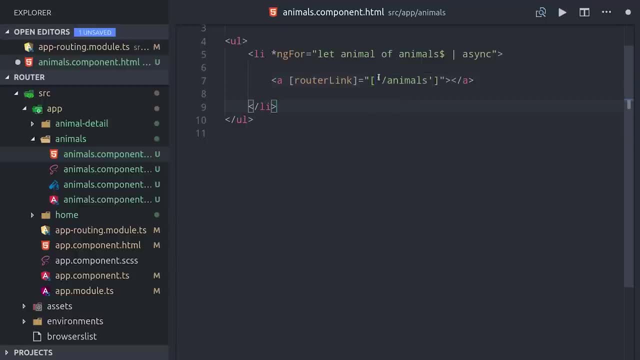 each item in that array represents a URL segment. So the first half of the segment is animals and the second half will be the animals. The parent component will need to tell the router where to render the child components, which we can do with a router outlet. 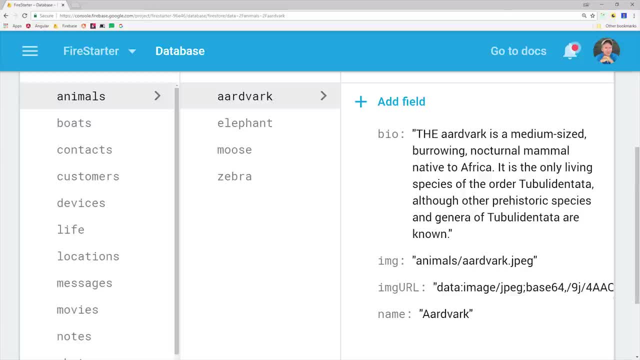 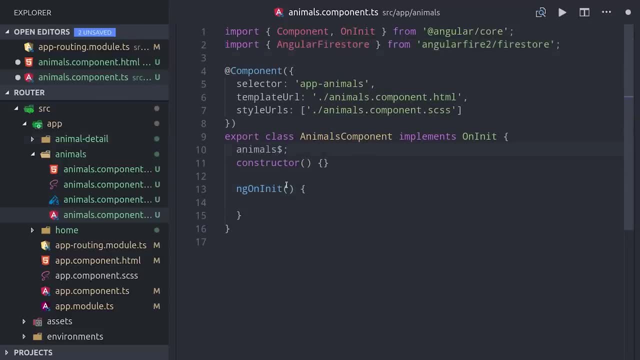 The actual data in the database is just a collection of animals that have a few properties on each document Inside the parent component. we can retrieve these documents with pretty much just a single line of code. we inject Firestore in the constructor and then reference these documents as the 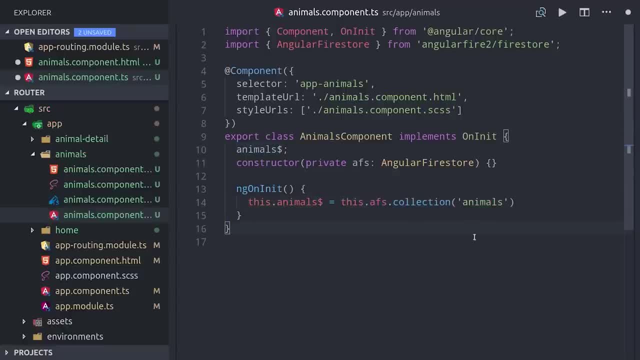 animals property and call value changes to listen to them as a real-time observable. In the child component Things are a little more tricky because we need to also listen to the change in the URL parameter to get the proper animal from the database. 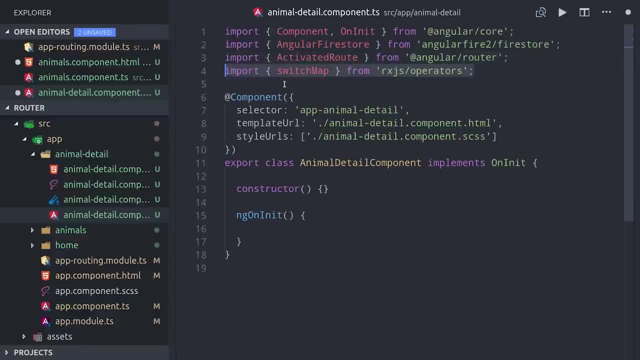 The angular router provides a service called activatedRoute that allows us to listen to state changes in the router, And then we'll also import the switchmap operator from rxjs. The important thing to understand here is that the component is only initialized once, when the first route is navigated to. 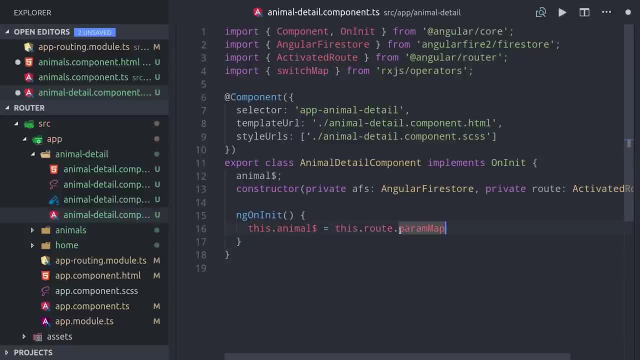 Any child routes that are navigated to after that won't be called with ngOnInit, So what we want to do here is use activatedRoute to listen to changes in that URL parameter, which is the animal's name, Which we can do by calling routeParamMap, which returns an observable of the route parameters. 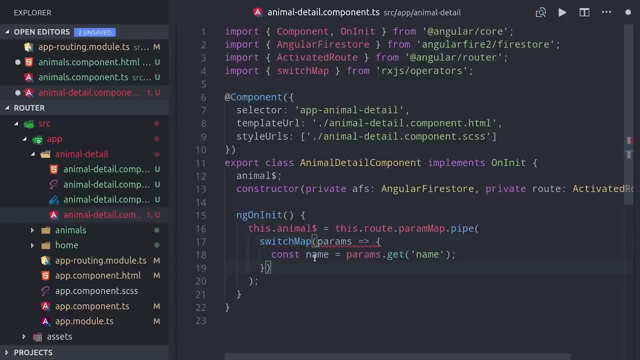 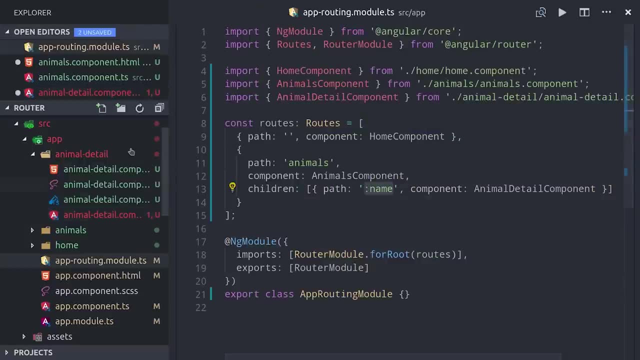 Then, when a change occurs, we'll call switchmap to switch to an observable of the actual animal data from Firestore. Notice how we're calling paramsgetName, which matches the dynamic URL segment that we set in the router config, So that returns the actual name of the animal, which we can then pass on to Firestore to. 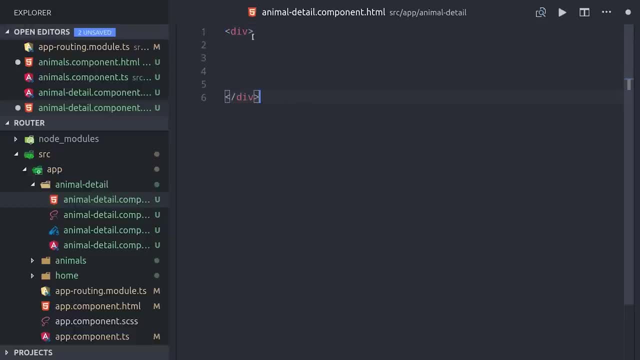 retrieve as a single line. The last step is just to unwrap this document in the child component, So we can do that with ngIfAnimalAsync. Then set that as a template variable of animal And we'll just show some of the properties here in the component, such as the name bio. 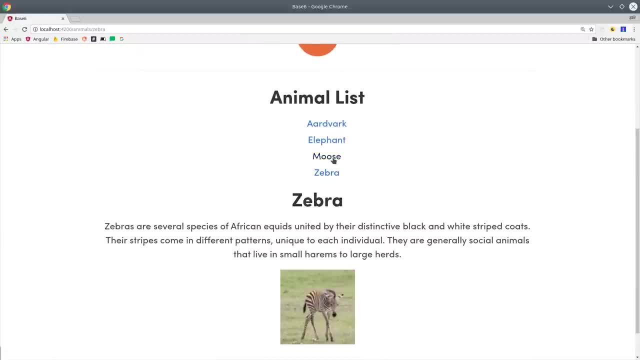 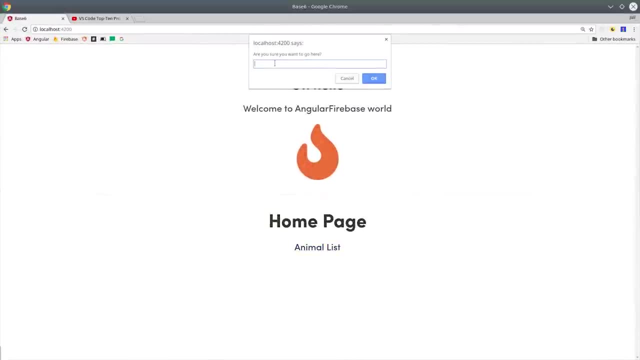 and image, And you now have a structured router tree that will scale up to as many documents as you have saved in the database. Up until this point, we've only been using router links to navigate, but you can also navigate directly from inside of the component's typescript. 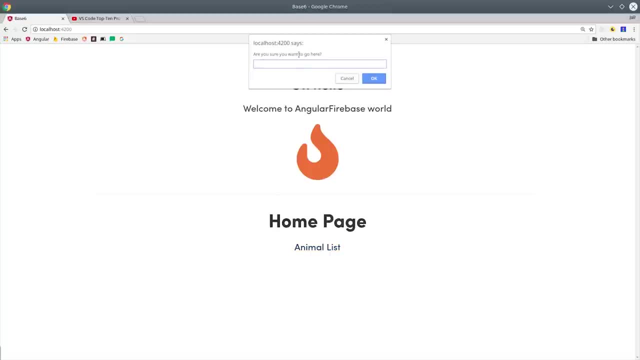 There are many cases where you just can't use it. You just can't use a link click to navigate to a page and you want to do it in a more dynamic way. Maybe you have some really ugly animals in your database and you want to prompt the 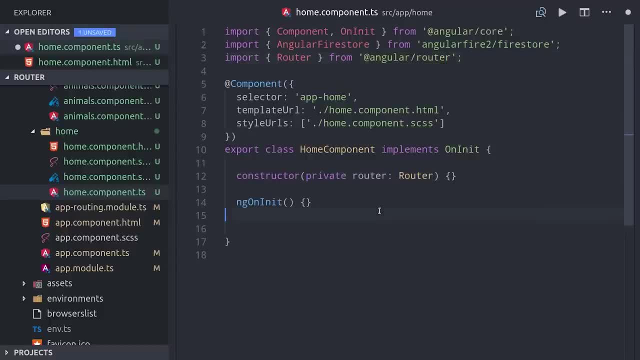 user to say yes before navigating. In this case, we will import the router directly into our component. We'll set up a click handler here that will first prompt the user to confirm that they want to navigate to this page and then, if they type in yes, we'll go ahead and navigate. 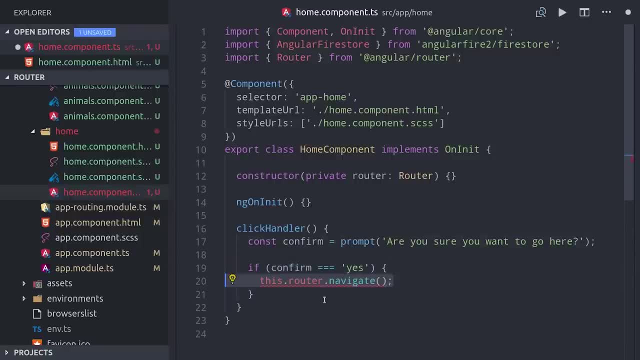 to that page manually with the router. You can say routernavigate and have it go to the array of URL segments that you point it to Using the HTML. we can go ahead and remove the router link and replace it with the click event that will run our click handler whenever it's clicked. 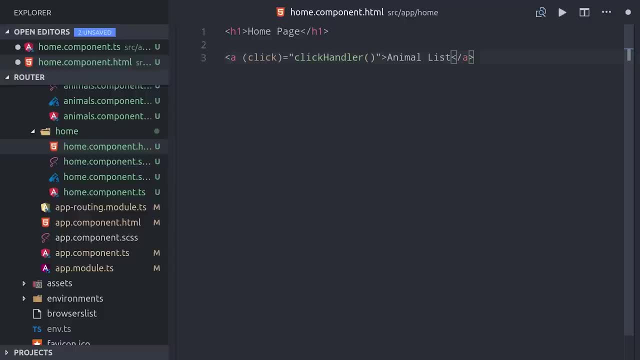 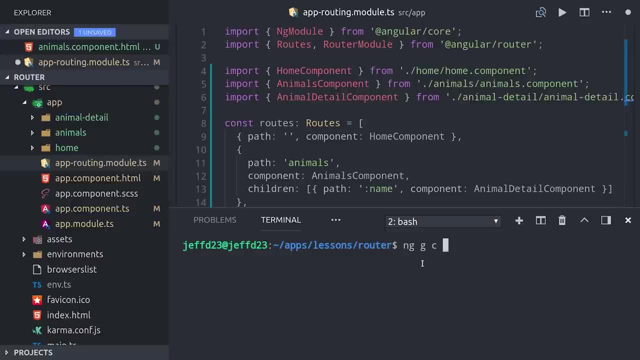 So the key takeaway here is that you can navigate anywhere in your Angular code outside of the scope of a regular hyperlink. Now I want to go ahead and switch gears and show you a couple things that are just super useful to do with the router. Let's say you want to create a catchall route that will serve more or less as a 404 page. 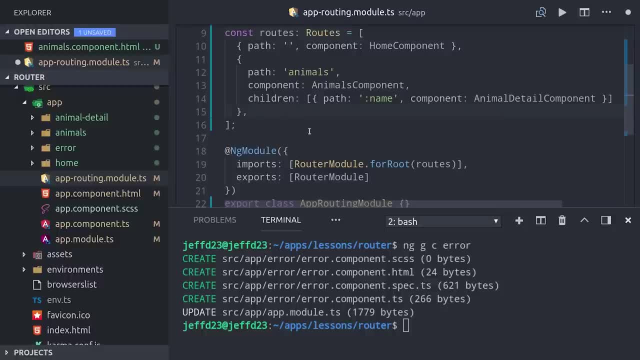 if the user routes to a component that doesn't exist, We can generate a new component to show the content And then we'll say pathnavigate, And you'll want to make sure that this route is the very last route in your tree. Then if we go and type in some random URL into the browser, it's going to pull up our 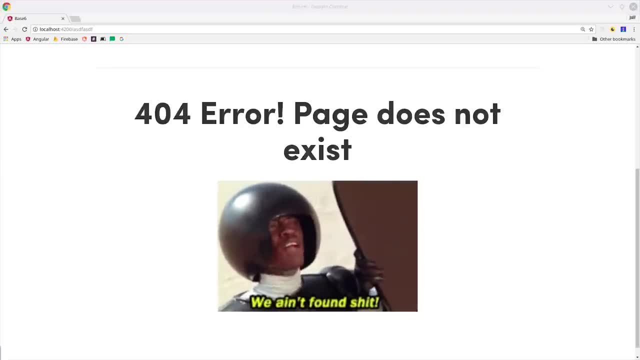 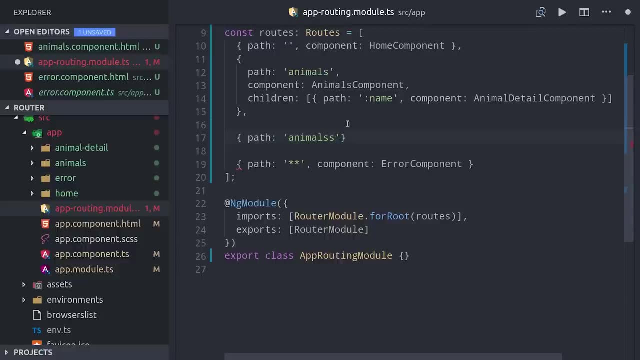 error component instead of just throwing a regular error to the end user. Then another very common thing you might want to do is, instead of routing to a component, you might just want to redirect to a different route. So let's say we have a common misspelling for animals. 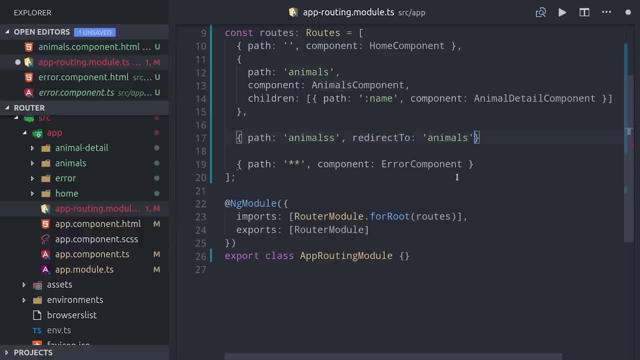 We can just redirect to the main animals route. When you set up a redirect route you'll have to also add in the path match option, otherwise the compiler will throw an error. If we go and navigate to this route in the browser, you'll see it redirects us to the 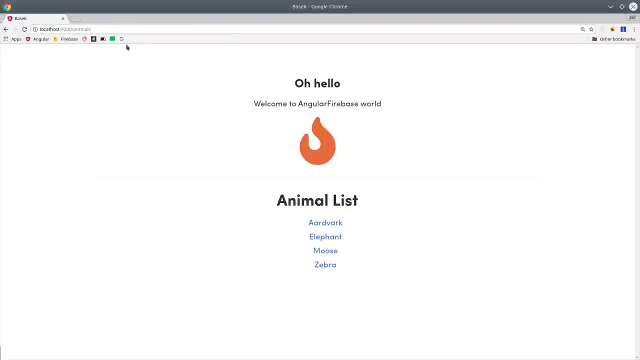 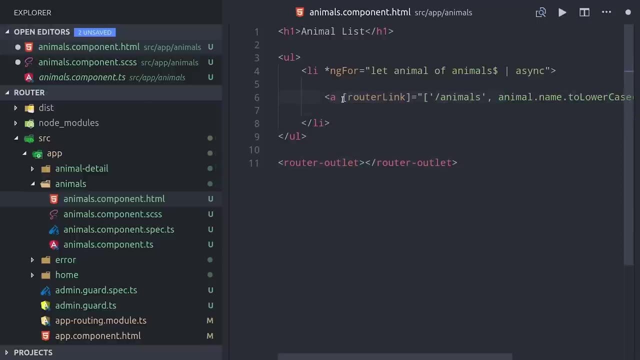 animals component, instead of bringing up the error component that we just created. Another cool thing you can do is use the router link active directive to provide a CSS class whenever a certain route is active. This makes it really easy to build out UI features that show the user which link they're. 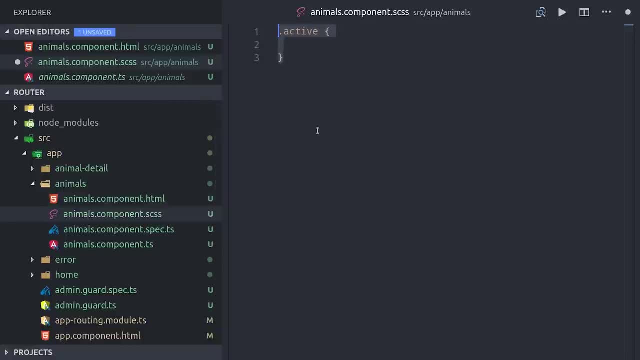 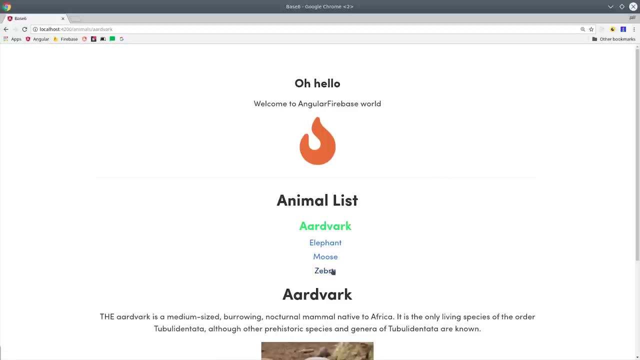 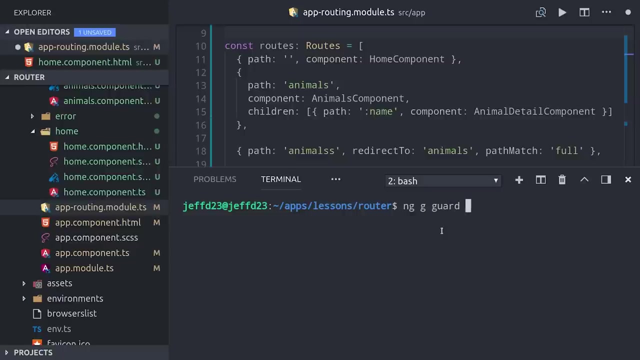 currently on. It expects a list of CSS classes on the right hand side, so we'll define an active CSS class field and a different color. Now you can see we get a clear UI change every time we go to a different link. For the next few minutes, I want to move a little beyond the basics and talk about guards. 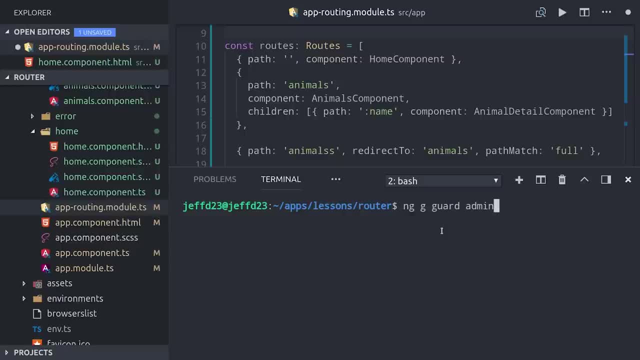 to protect routes, create reusable code and preload data into your components. A guard is just an Angular service that has some special interfaces that we can implement to do things with the router. One of the most common use cases is to protect routes from unauthorized users. 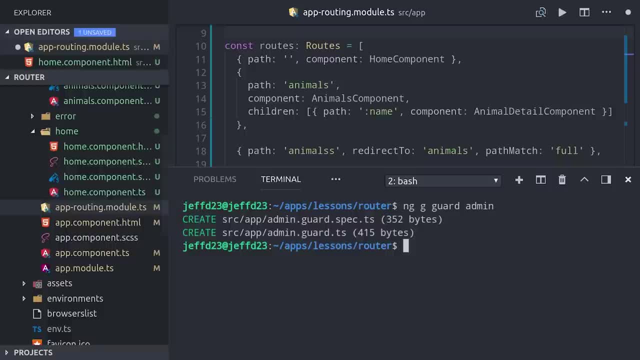 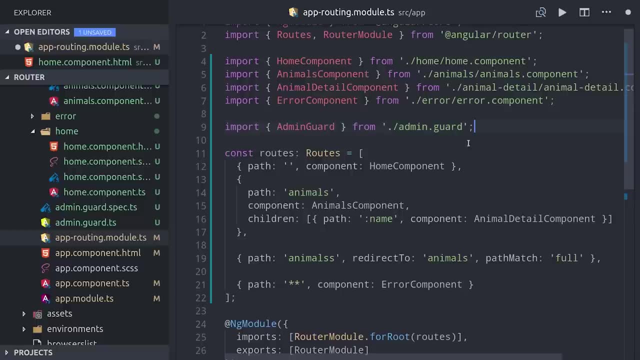 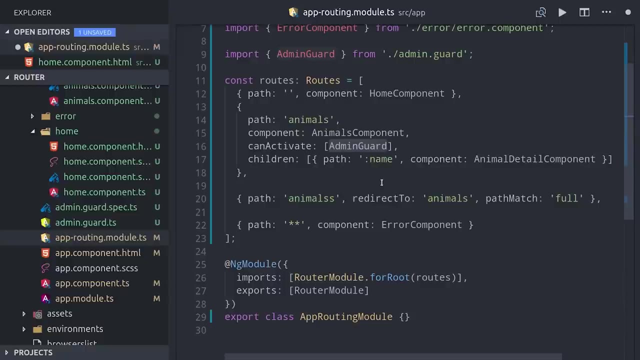 Let's go ahead and run ng generate guard admin. that will protect our routes from any non admin users. The special interface we'll be using here is can activate, which will only activate this route if the guard resolves to true. Let's go ahead and lock down our animals route by adding the can activate property with the 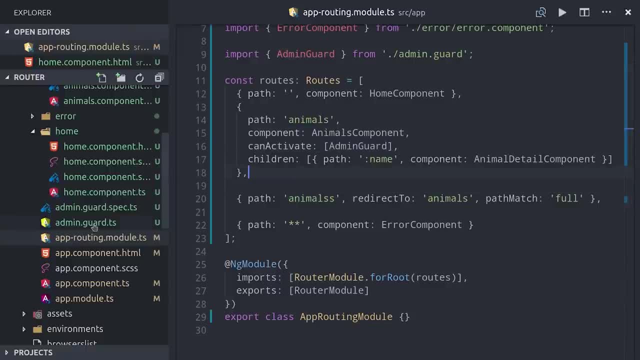 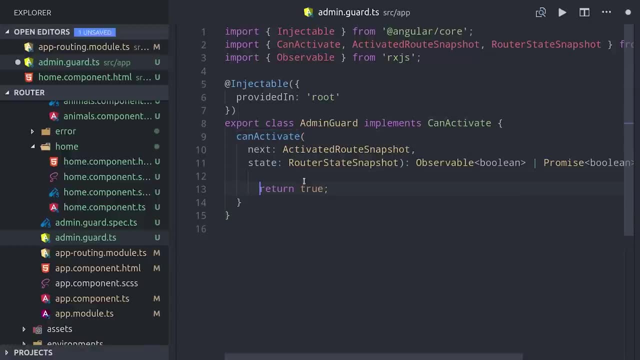 admin guard. If we go into the guard itself, you'll see that it is decorated with injectable, just like any other Angular service. The only special thing is it has this can activate interface that gives us some information about the state of the route. 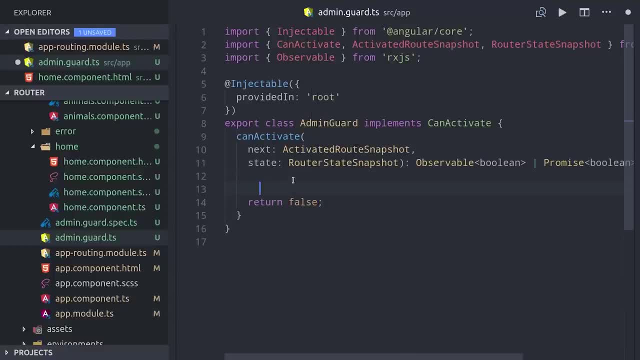 In order for the guard to work, we just need to return a board. This can be boolean, which can be a primitive, or it can be an observable or promise. If it's an observable, it's going to automatically subscribe for you. 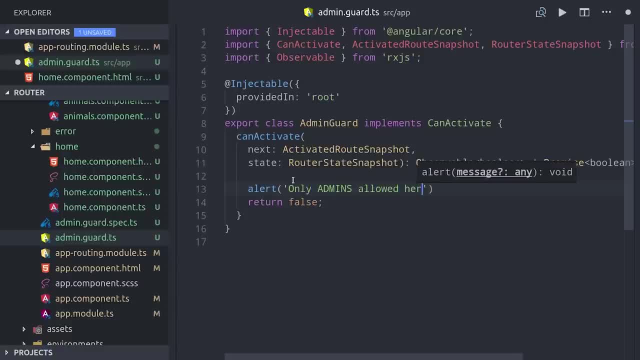 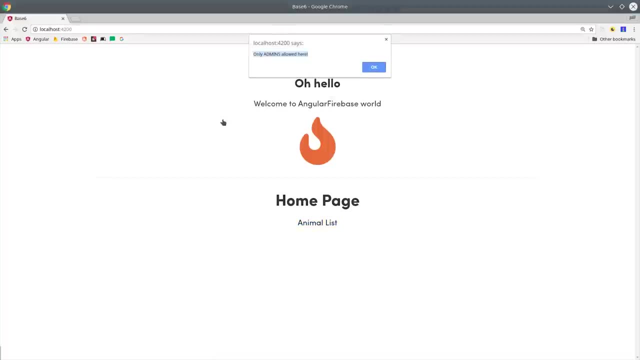 So we'll go ahead and send an alert that says only admins allowed and then we'll return false to block access to this route. If we try to navigate to the animals page, you can see we get this alert and the component is never rendered. 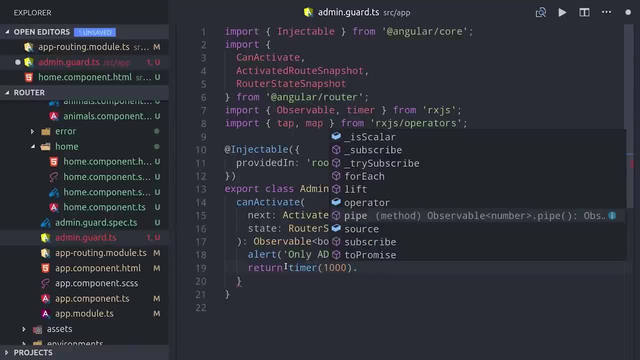 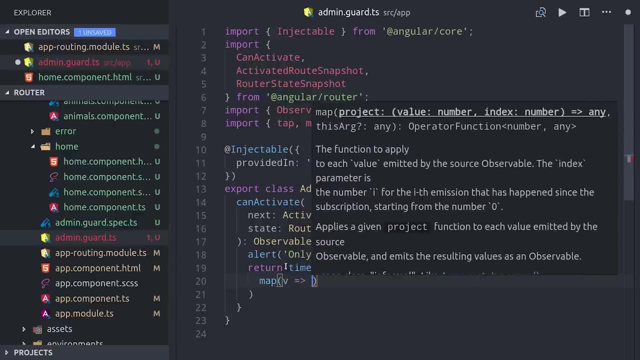 But more often than not you'll need to do this asynchronously by checking with some API if this user has authorization. We can simulate this by setting up a timer of 1000 milliseconds. Then we'll need to map the emitted value down to a boolean. 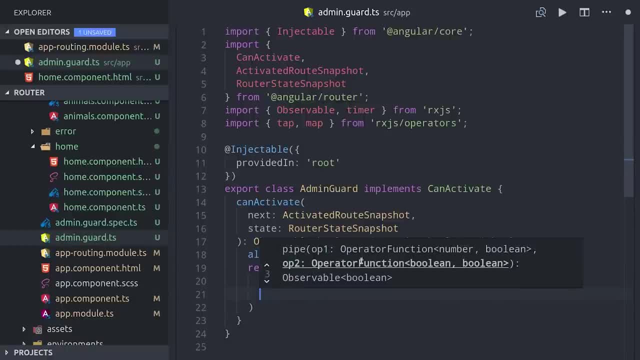 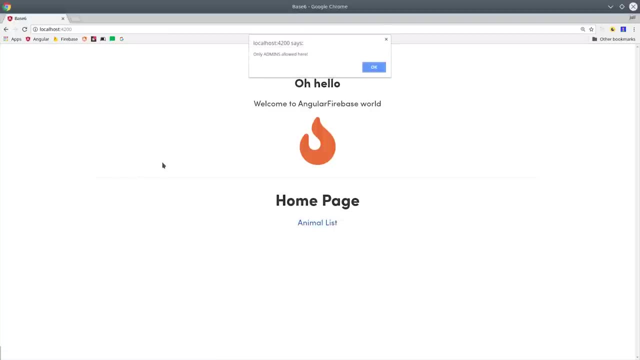 Then we can also use the tap operator to show an alert or this is a good place to navigate to a login page or something along those lines. If we try to navigate to the page this time you'll see we get a one second delay and 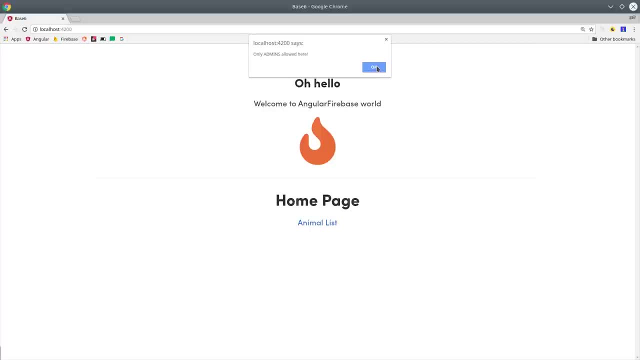 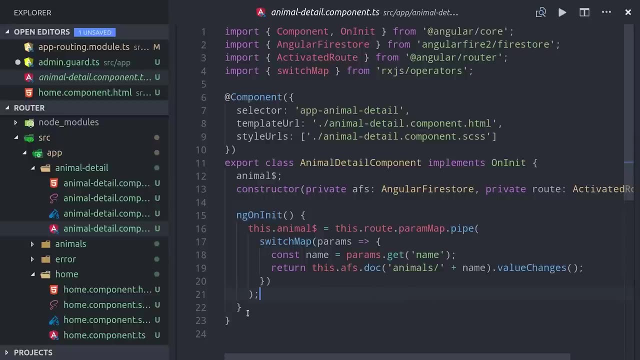 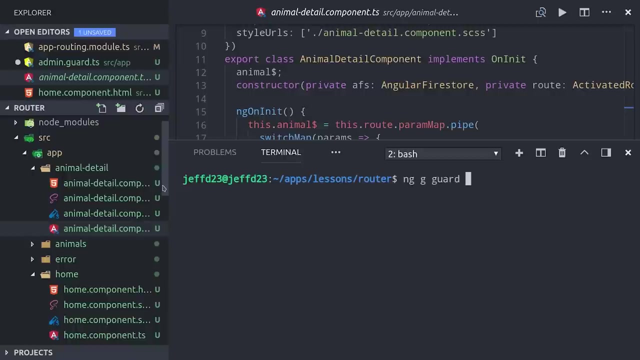 then it finally blocks the route. after this observable is resolved, Can activate is a very powerful interface at your disposal, but there's also another one called resolve that can preload data into your route. Do you remember earlier how in the animal detail component We listened to the name parameter and then switch map to a different observable? 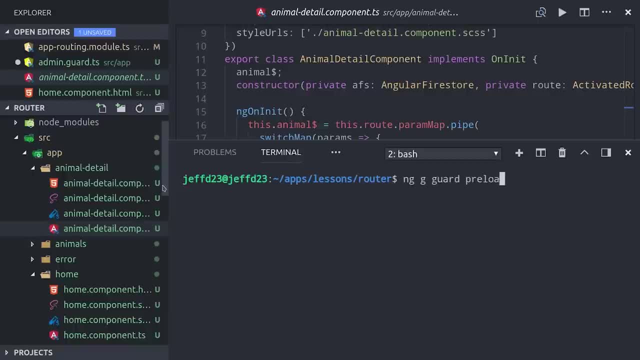 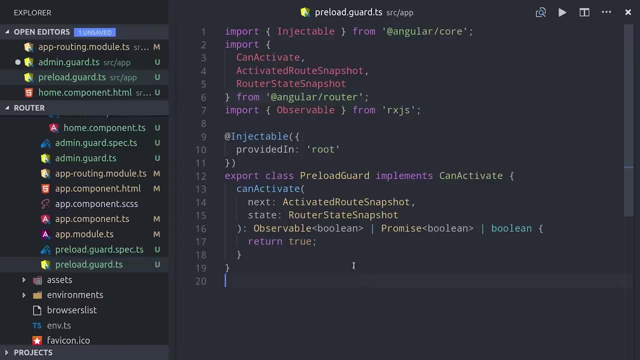 Well, maybe there's a better way we can do this. Imagine we wanted to preload this data on multiple different components. We would have to write this code for each one of them. Instead of repeating ourselves, let's generate a guard called preload. Instead of using the can activate interface, we'll use the resolve interface, and you could. 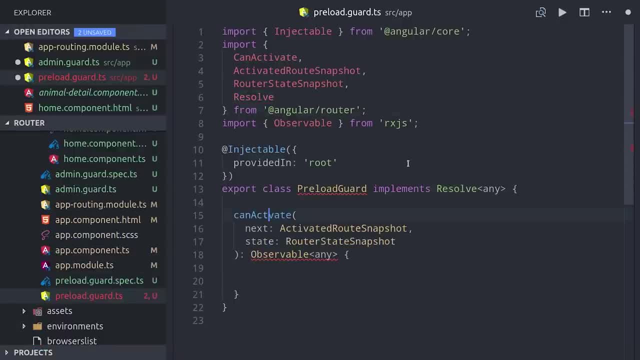 strong type this as well, but for now we'll just use any. Then we'll change the method name to resolve, and it's pretty similar to can activate, but instead we'll return the actual data that we want to be And commonly that's going to be an observable form, because you're probably pulling this. 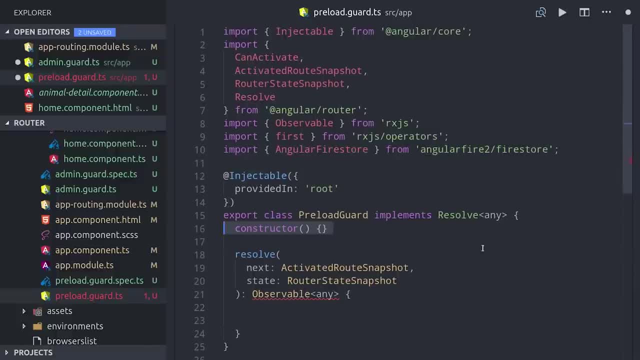 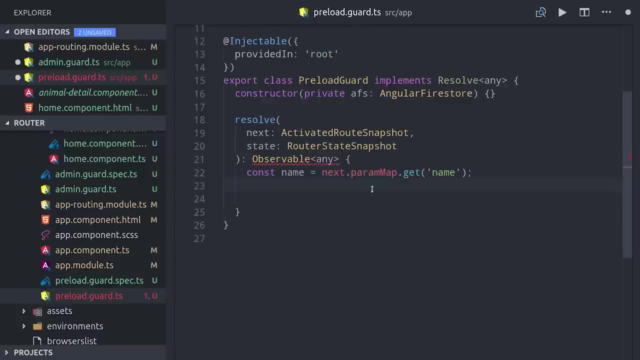 data from some external API. In our case we'll do it with angular firestore, so we can inject that in the constructor. Then the guard will have the actual parameter name available as a plain object which we can retrieve with nextparammapgetname. 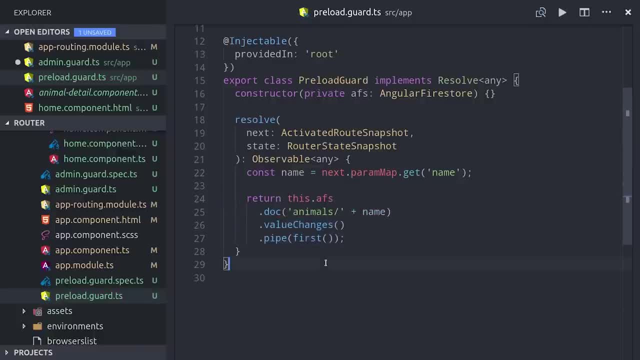 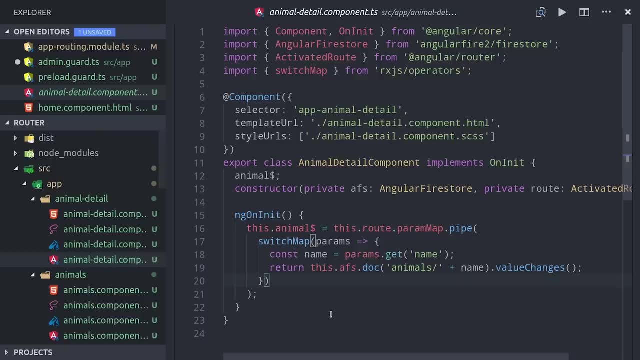 Then we can just return the data as an observable, but we have to pipe in the first operator, because firebase returns real time stream. We need this observable to be available when this route is navigated. Now we can just comment out all of our previous code and instead we'll just define the animal. 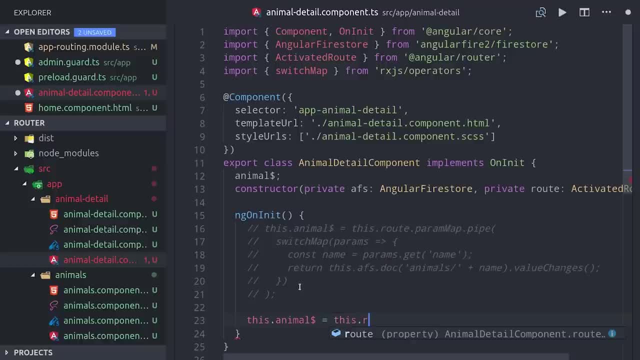 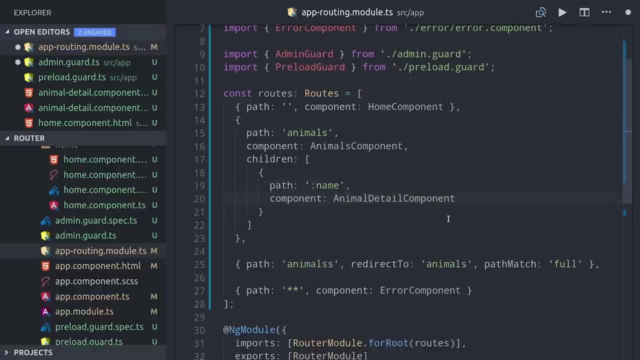 as the data that is now available on this route when it's navigated to, It's now available on the route data property and then we can apply it to this route by going back to our router config. then add the resolve property to our preload guard. 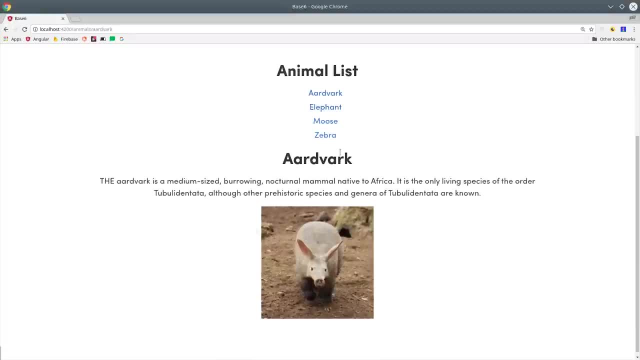 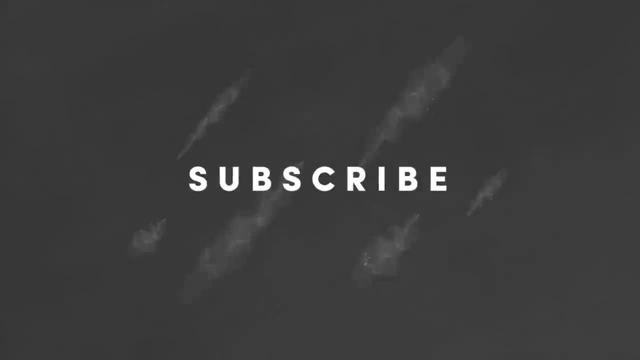 If we open up the app, it's going to work in exactly the same way as it did before, but now we've isolated this code in a reusable way that we can apply to multiple routes as needed. Hopefully that gives you a basic idea about how powerful the angular router can be. 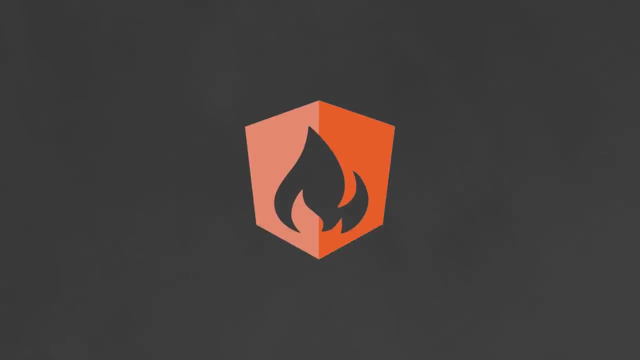 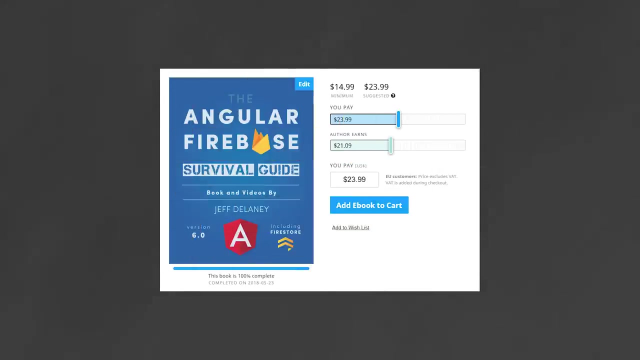 I'm going to go ahead and wrap things up there. If this video helped you, please like and subscribe. and if you really want to master the basics of angular, consider becoming a pro member at angularfirebasecom. You'll get access to a whole bunch of exclusive content designed to help you build and ship.